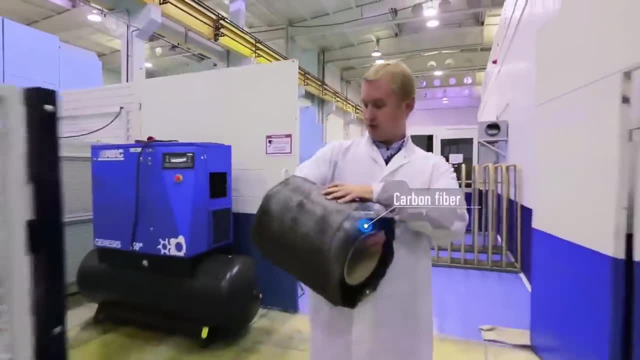 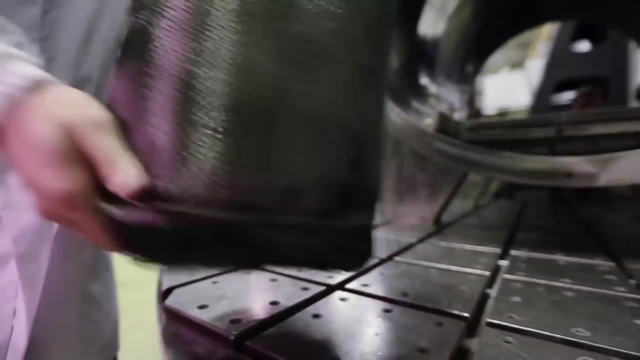 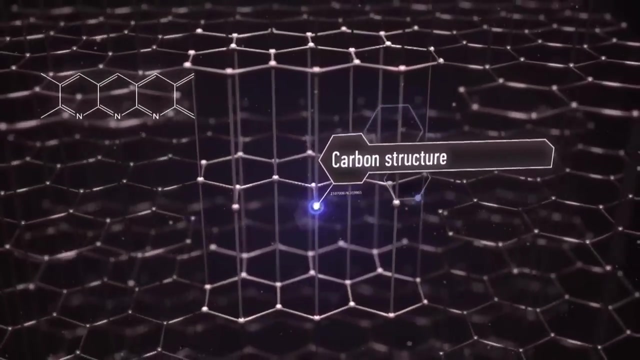 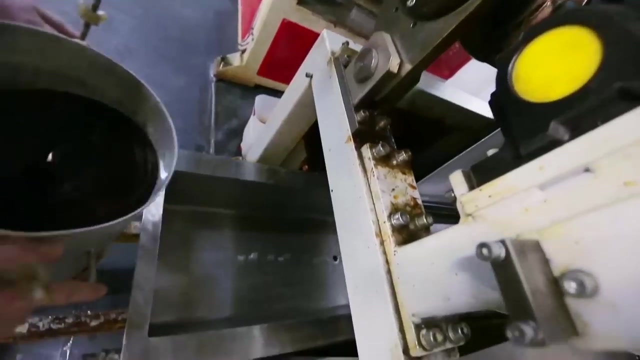 it is this sort of carbon material. It feels soft, but it will later become a stiff spacecraft skeleton. The idea behind carbon plastic is using carbon fibers into weaving a carbon fiber fabric. The fiber is submerged in a binding solution. usually it's epoxy resin. 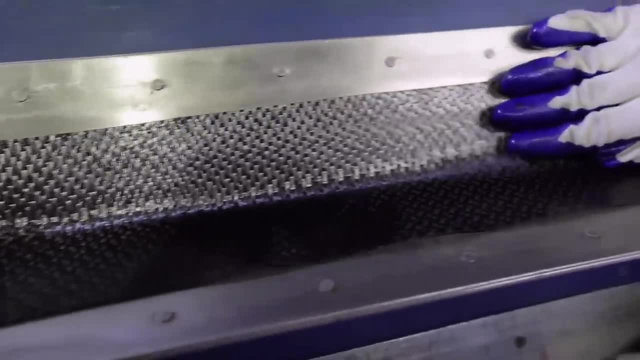 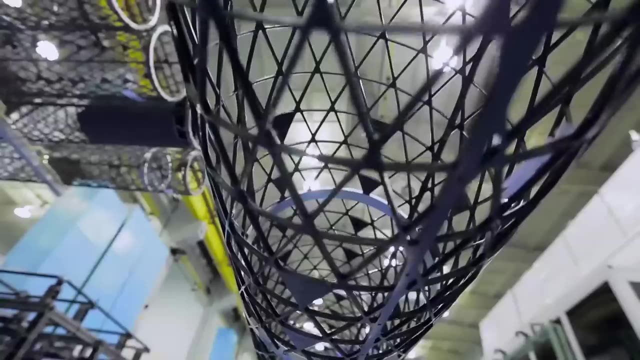 The material is later shaped with the help of a knife and a matrix. Then we let it dry and voila, here's a part of a future satellite. The weight of the carbon fiber parts, of course, is extremely important. This is a future satellite. 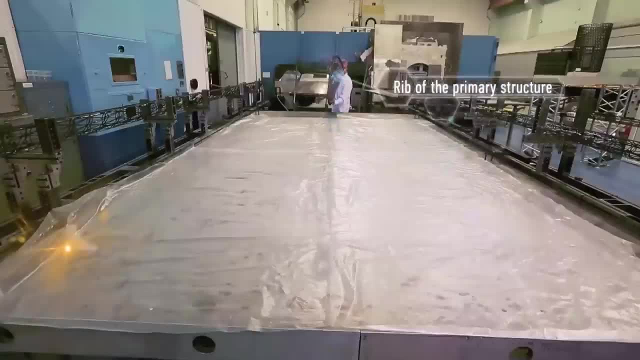 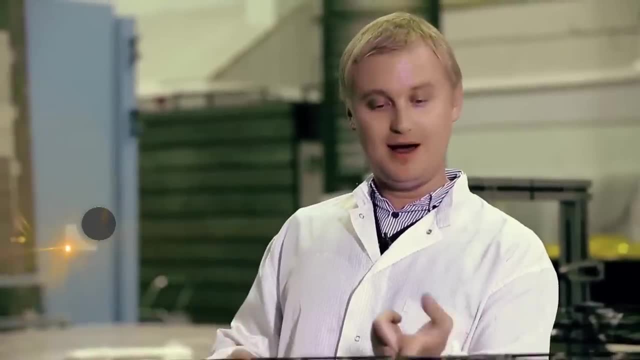 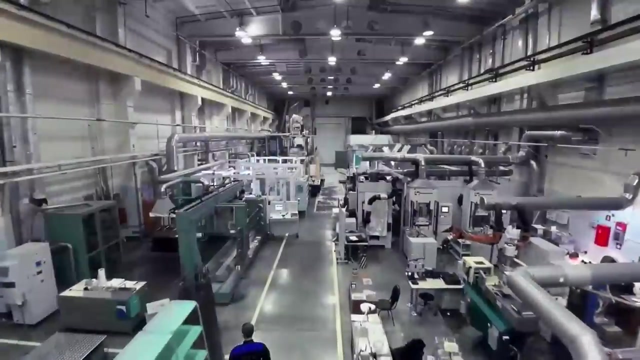 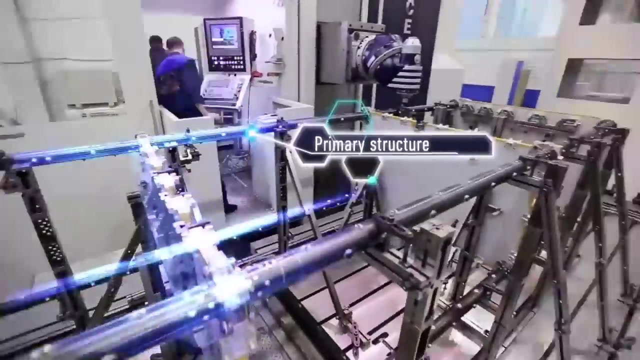 antenna pole, An extremely sturdy thing. It's 6 meters long. You can lift it with your left hand. Actually, a finger of your left hand will do the job. The assembly of a carbon fiber component of a communication satellite starts at the milling center. we start with the 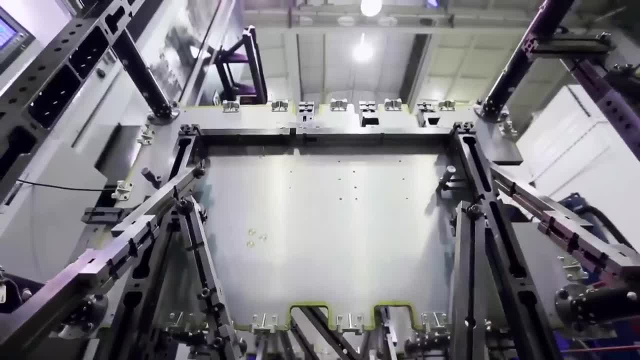 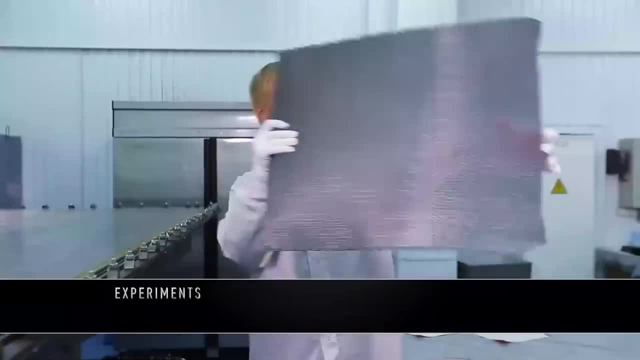 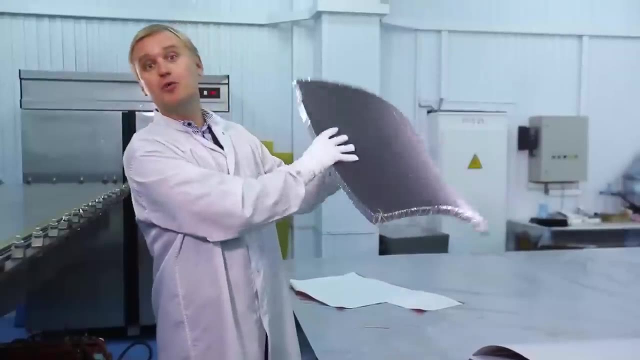 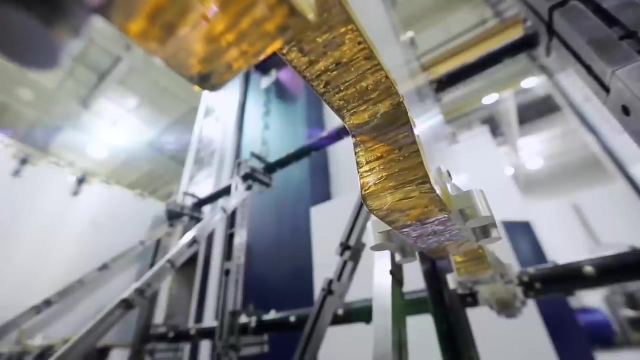 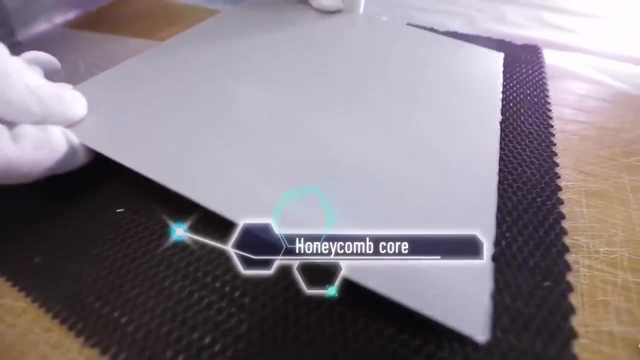 carbon fiber primary structure. then we attach honeycomb panels. here's our future body frame. to an amateur it may seem: well, what kind of a frame is? this must be a joke. oil cells- it's wobbling. what's dirtiness or stiffness are you talking about? the key here is the top and the bottom of the sailor foil. it is. 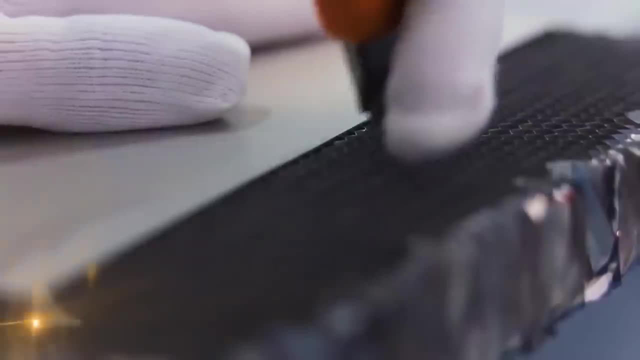 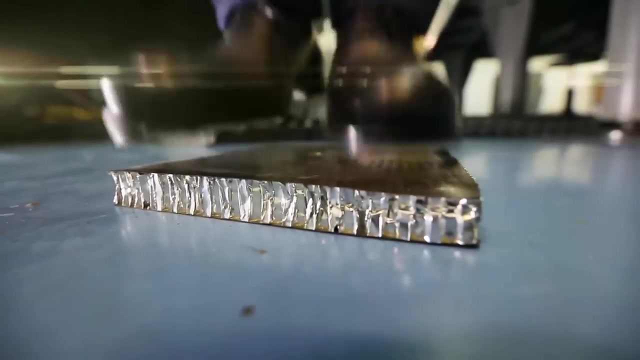 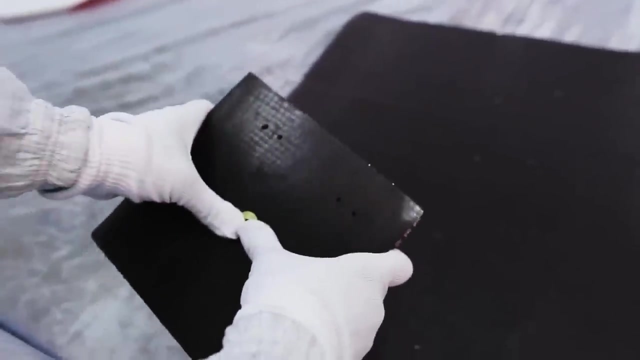 called the honeycomb core, by the way, is reinforced with aluminum or plastic plates. the core turns into a stiff frame after it dries- very stiff and very light. same principle with the bottom of the cellar foil. the bottom of the cellar foil is in carbon plastic. the future spacecraft parts must be both durable and light. 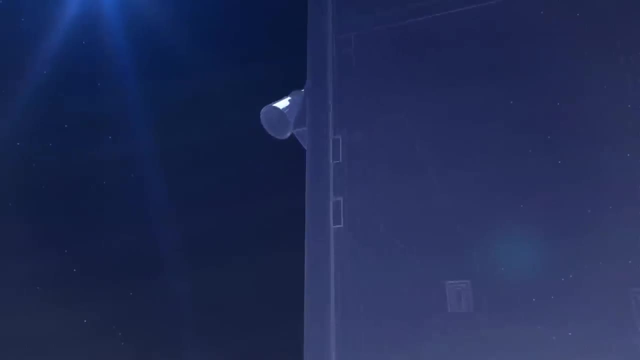 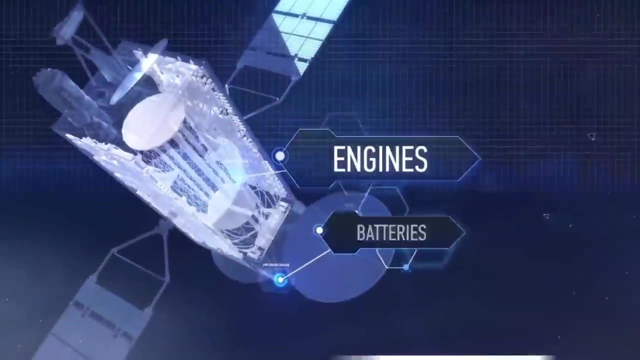 why is it so important to cut weight? any satellite consists of two big parts: a service module and a payload module. service systems consist of engines, batteries, solar panels, incomm. Goodbye. This is the American. genauing tastes like a Pinch myTO, clippers and scissors. aBE a wanted going ahead and taking a chock of. 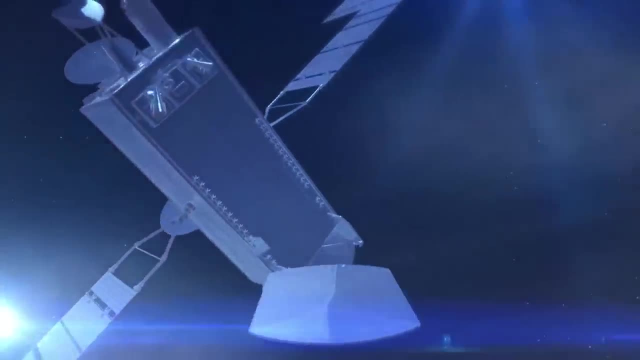 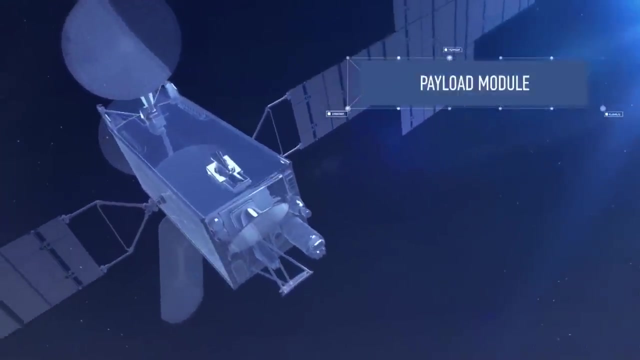 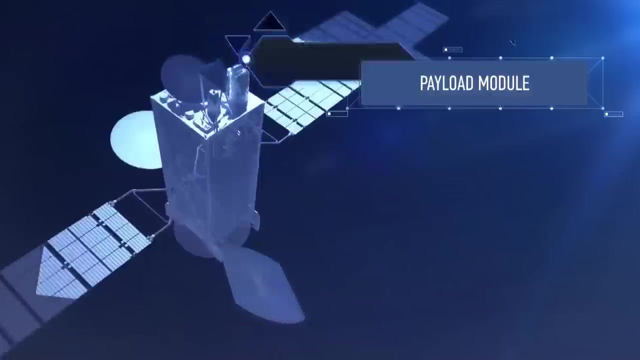 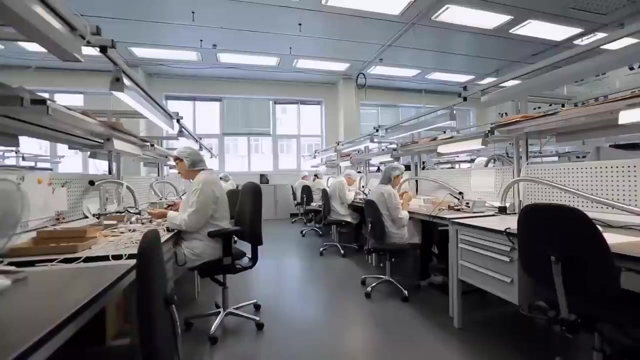 panels. whatever is required for in-orbit operations, the payload is the reason the satellite is in orbit. the tools, for example, communication satellites need antennas and transponders. therefore, the lower the spacecraft weight, the more payload it can carry. there is a direct correlation between the two, as in any 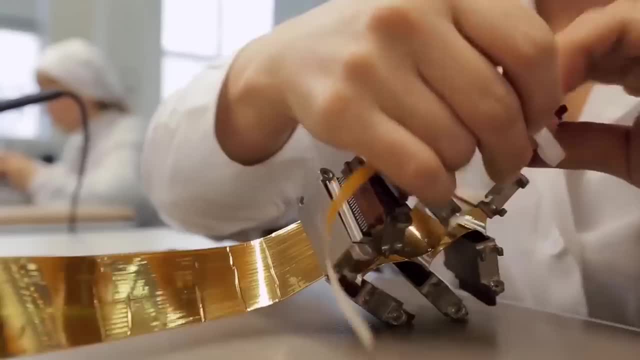 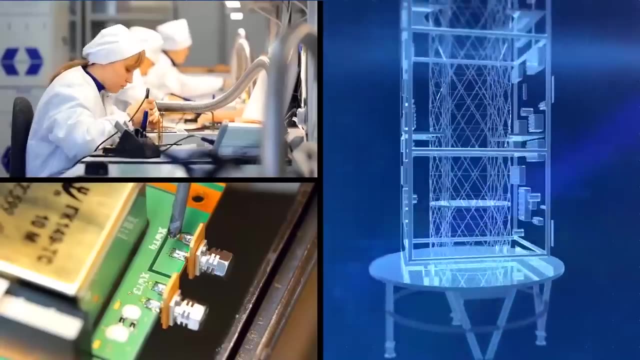 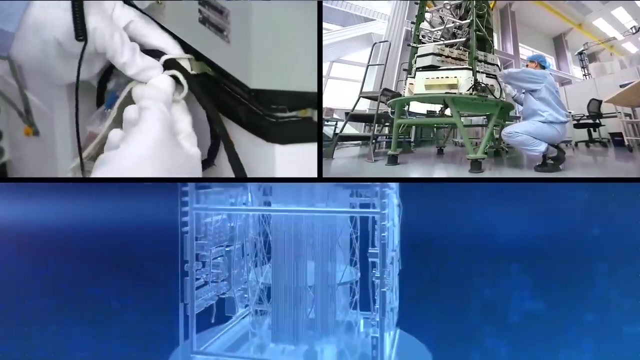 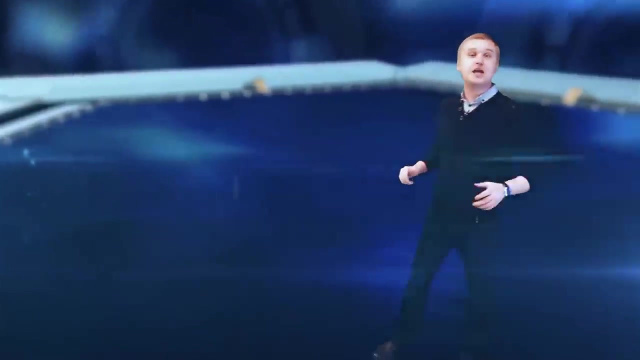 other electronic device, be it a phone or tablet. satellite microchips in satellites tend to get smaller each year. microchips are assembled into blocks. they are then attached to the frame. the communications satellite literally snowballs into what it's meant to be by adding new units and parts. in general, the spacecraft assembly. has very little to do with assembling. let's say, a car too many fundamentally different systems, that is, solar panels are built by one manufacturer, antennas by a completely different one, and often the service module and the payload module have different manufacturers as well. but manufacturing is one thing, assembling and testing is another. here's the reason. 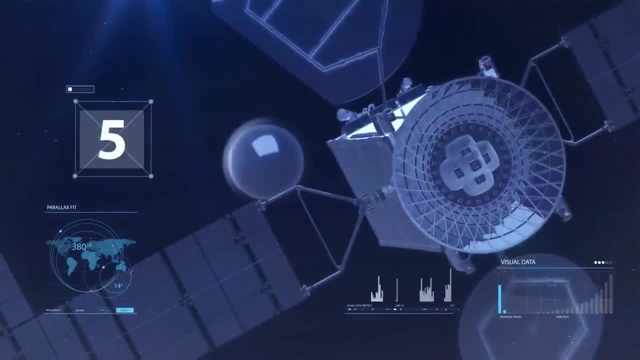 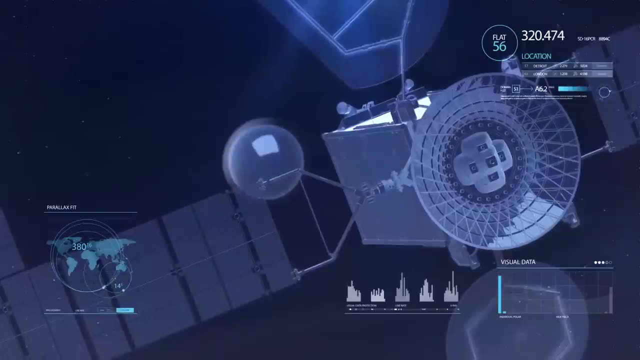 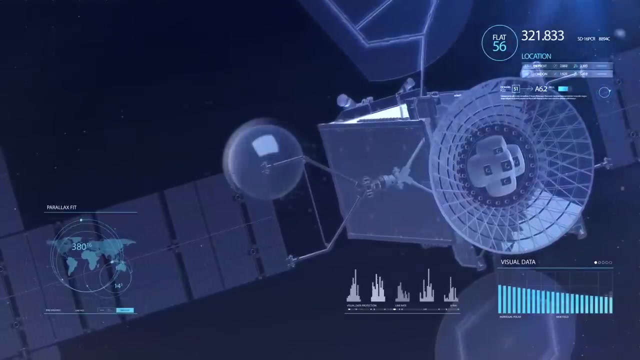 why communications satellites will have to function in space for 5, 10, 15 years, and if something goes wrong, we can't just send over a maintenance team. there's no such thing as maintenance for a satellite. therefore, we have to double check each unit and block to make sure they are durable, among other things. 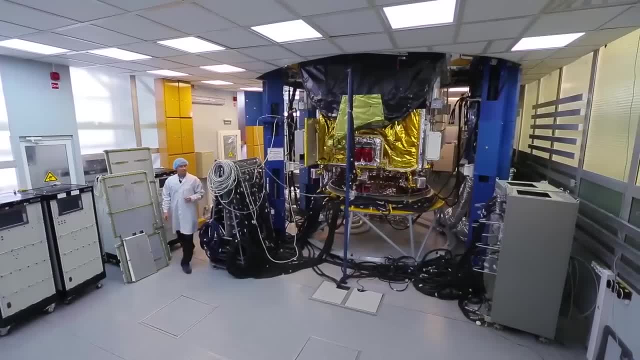 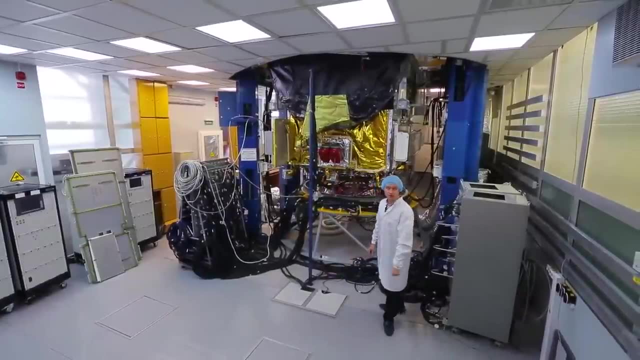 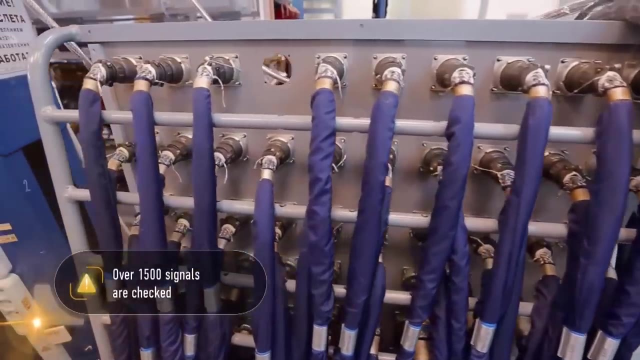 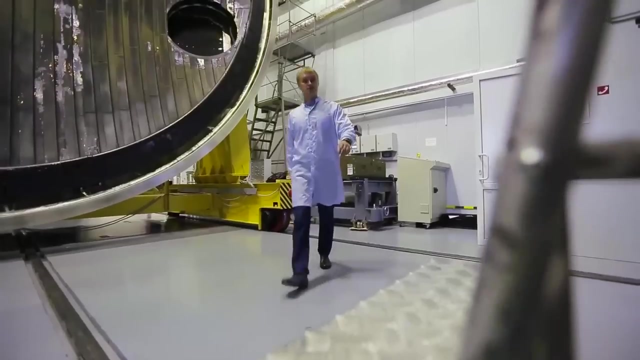 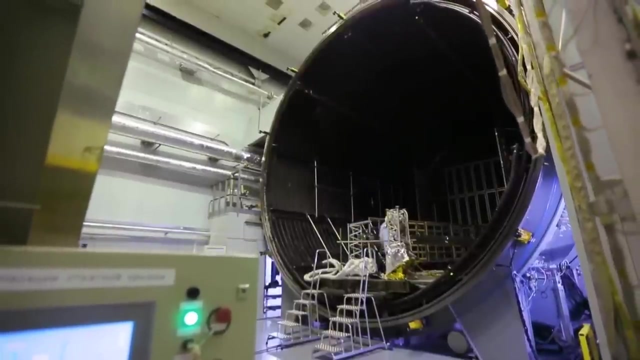 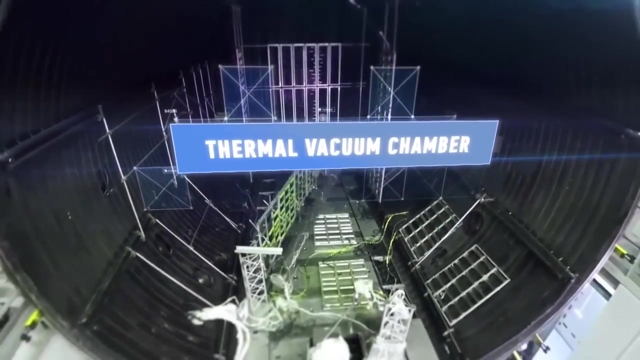 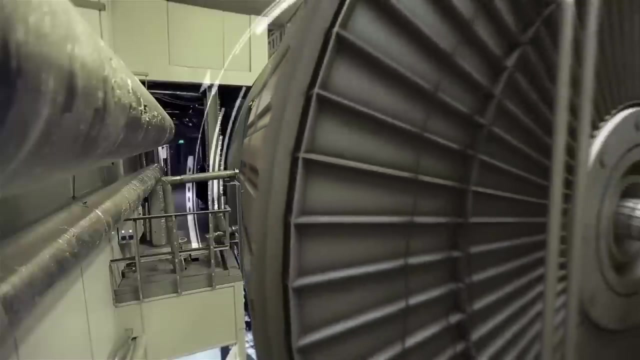 electrical testing is perhaps the most common test for any satellite, including communication ones. but in between electrical tests, a spacecraft undergoes a number of exotic durability tests. this construction is called a thermal vacuum chamber. during the test, the chamber is sealed, air is removed, creating a high vacuum inside, and then 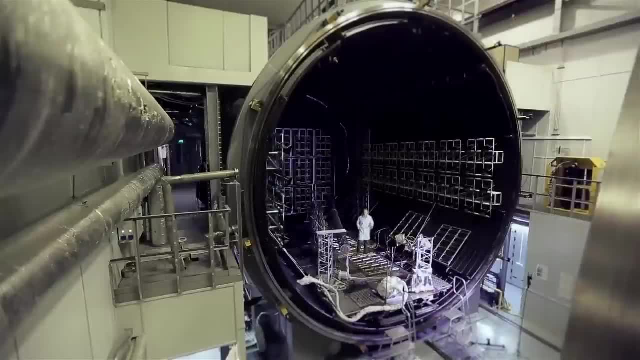 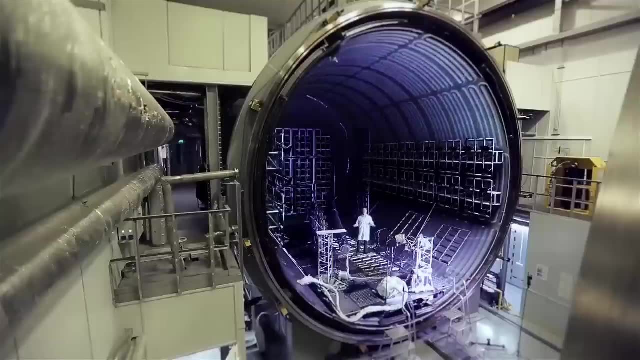 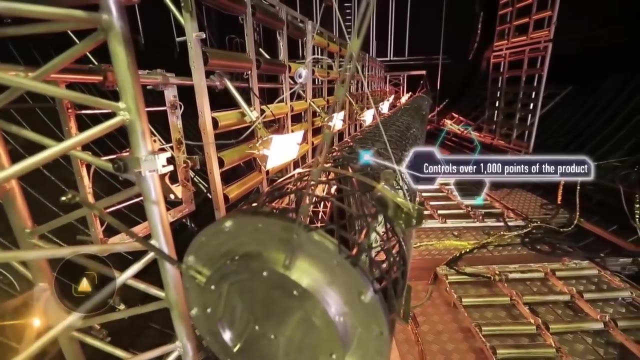 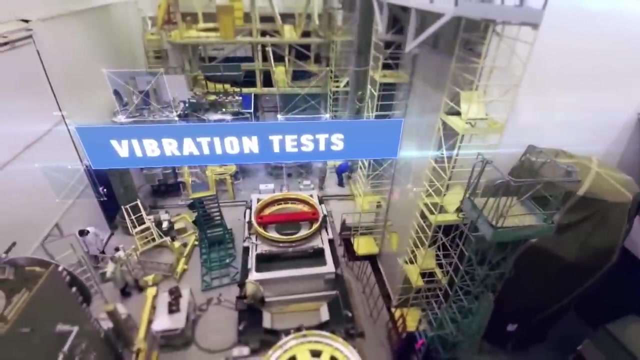 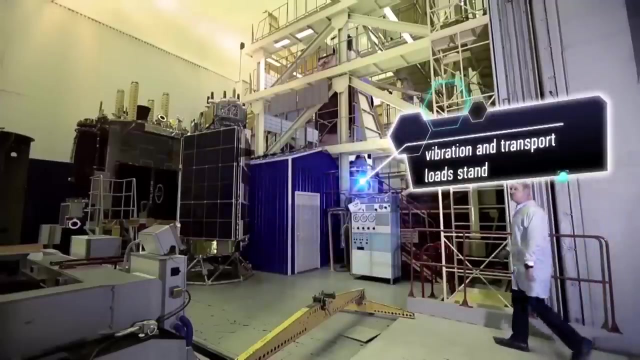 the temperature is alternated between plus 150 degrees Celsius and minus 150 degrees Celsius, thus assembling outer space. that is how experts test whether a communication satellite and its blocks can endure extreme temperature changes while in orbit and in the next room they tested, the satellite can make it to the orbit. this is a vibration and transportation loads testing stand. 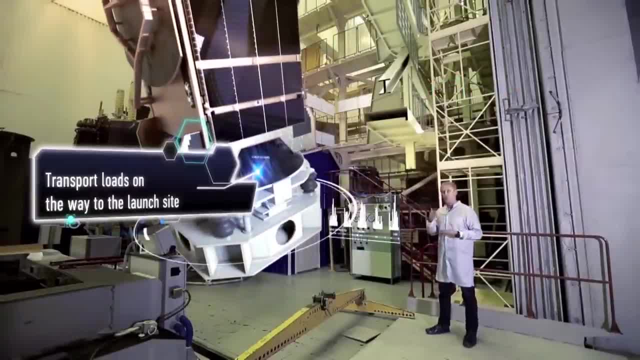 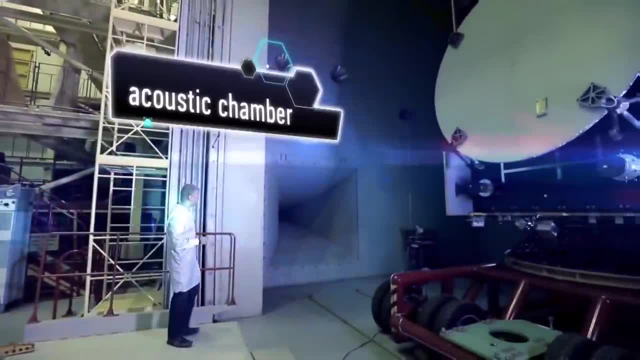 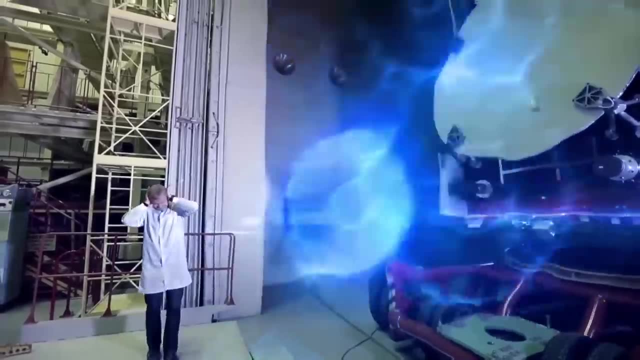 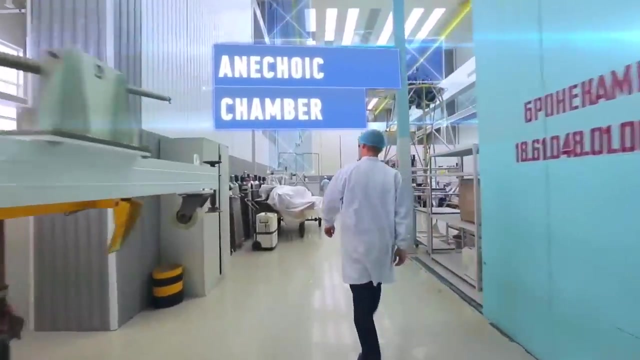 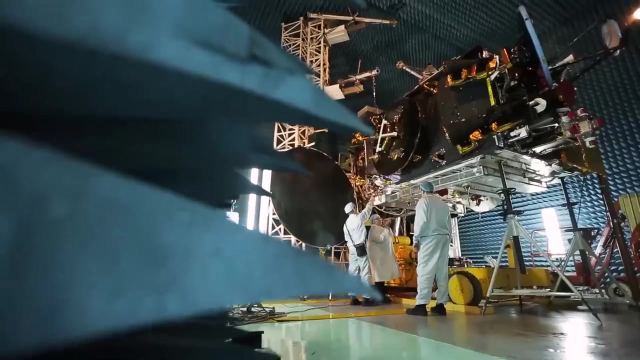 here we recreate the shaking conditions the satellites will undergo, first and foremost on their way to the launching site and later during the rocket launch- and this is an acoustic chamber. here the spacecraft will literally get deafened. the communication satellite is almost ready. there's one more important test: antenna testing. 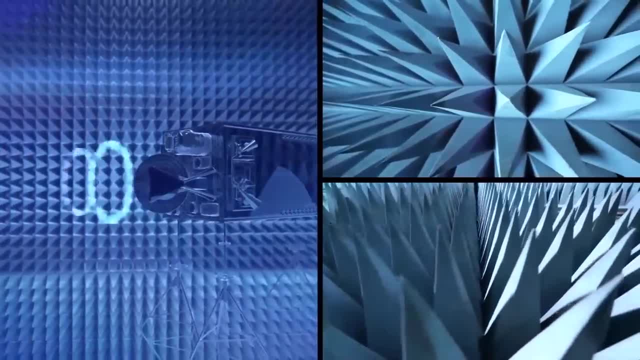 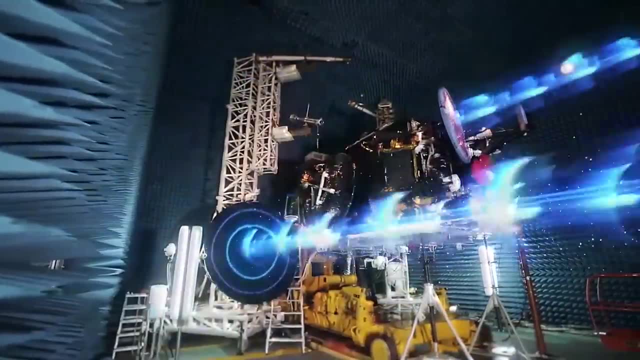 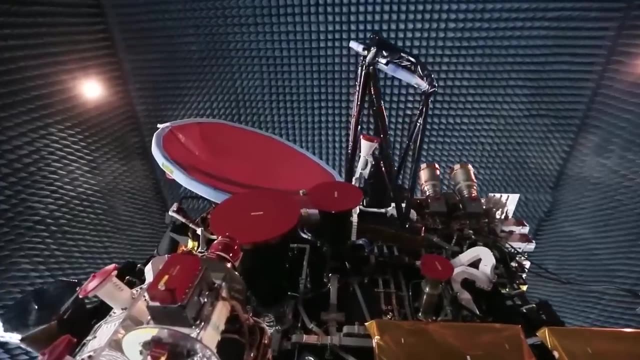 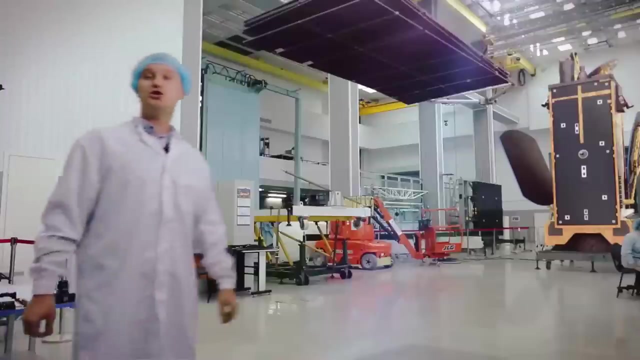 they are tested in an anechoic chamber. the signals here are not reflected back from the walls. everyone leaves the room during the test. too much radiation. if all goes well, the antennas will get locked down. they won't be moving until they are in orbit. one of the final stages of a satellite assembly is wing. 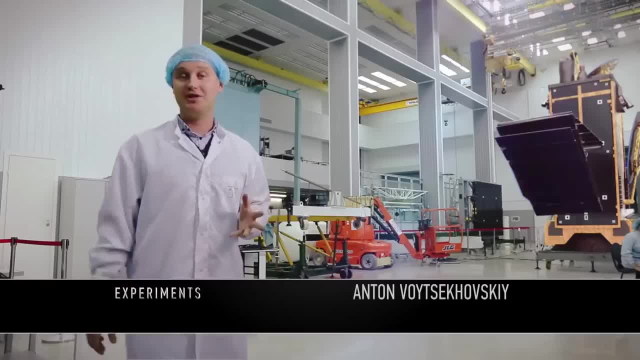 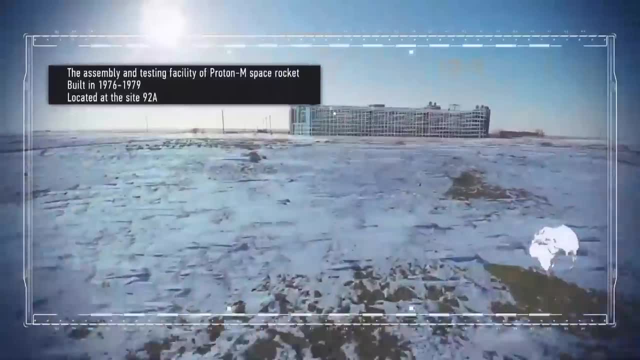 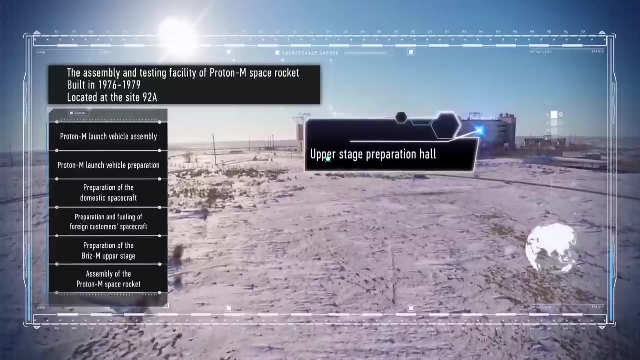 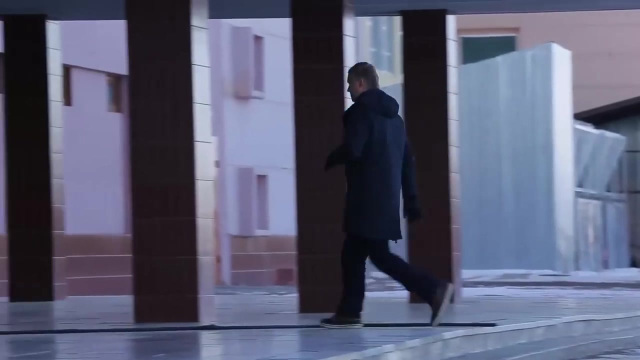 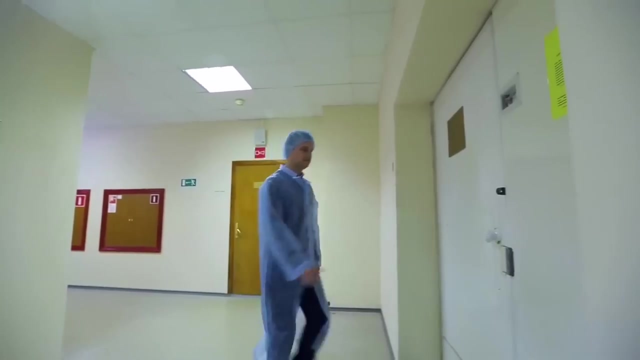 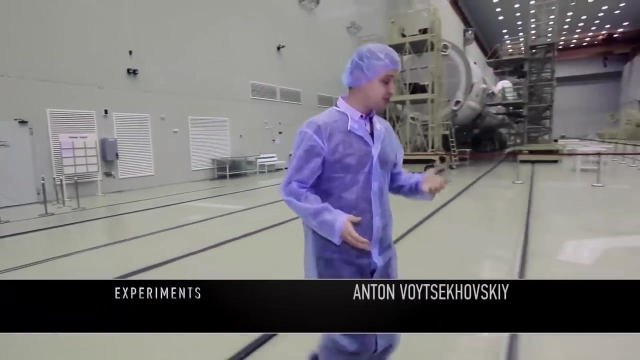 attached fittings: the wings system, solar panels. well then, there's only one thing left to do: transport it to the launching site. that's the building for this task, the assembly and testing facility, me. these facilities are a part of almost every spaceport, otherwise it is impossible to assemble. 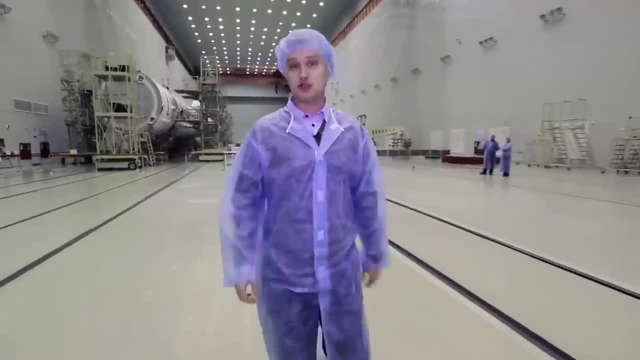 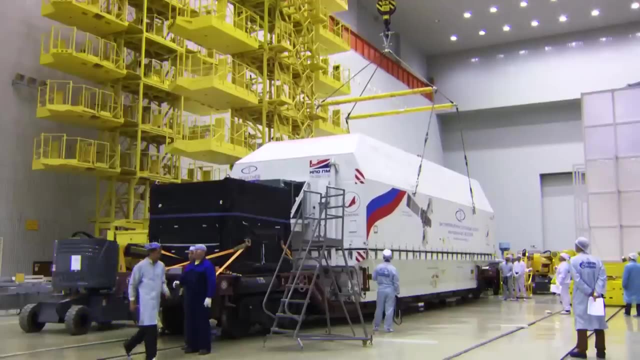 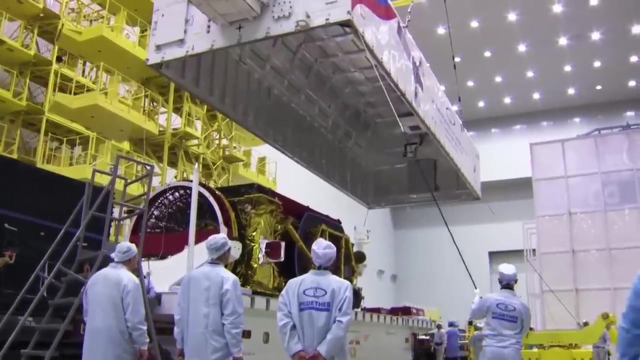 and test the launch vehicle and, most importantly, to made it with its head, the satellite. if the communication satellite arrives here in just one container, it takes 16 cargo cars to transfer the proton m launch to the launch site. the launch site is located in the center of the 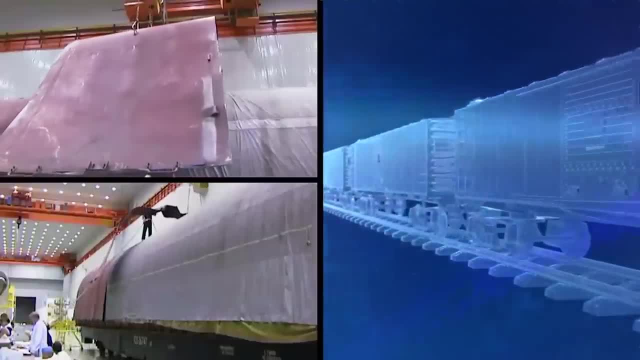 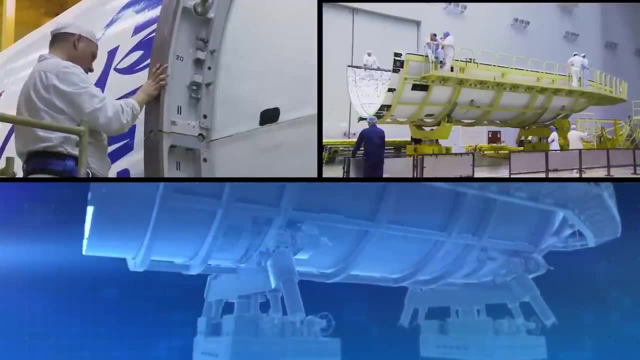 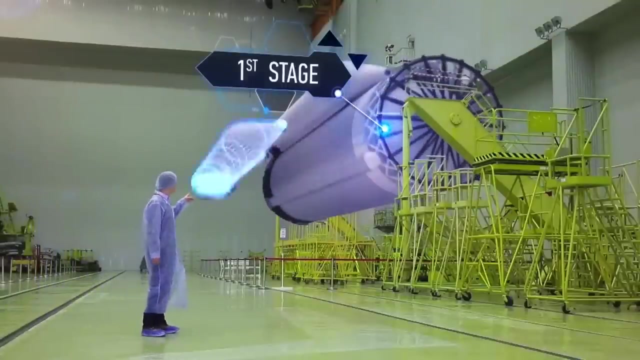 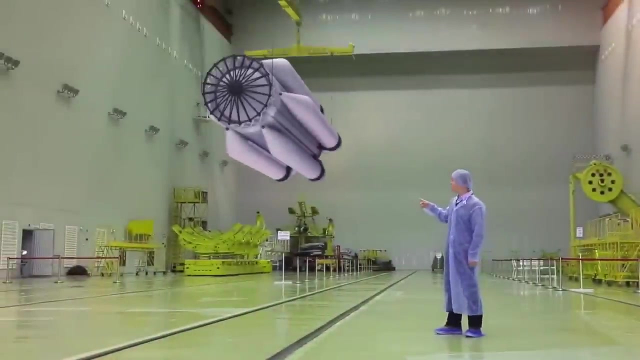 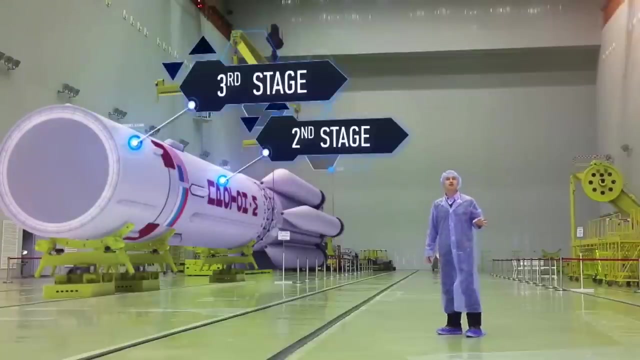 vehicle. now we can start assembling the rocket. the assembly of the rocket reminds one of a construction set. the first stage is assembled on this jig, then the first stage is transferred by a crane to that part of the facility and made with the second stage than the third stage. 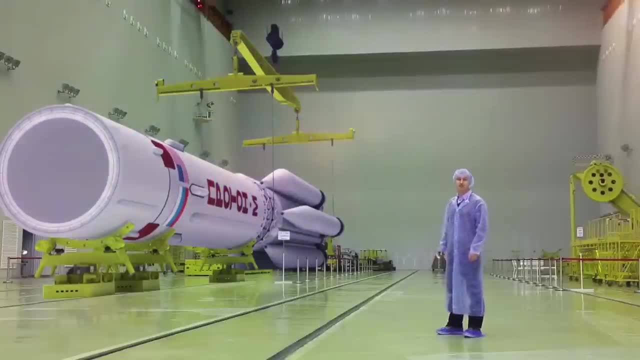 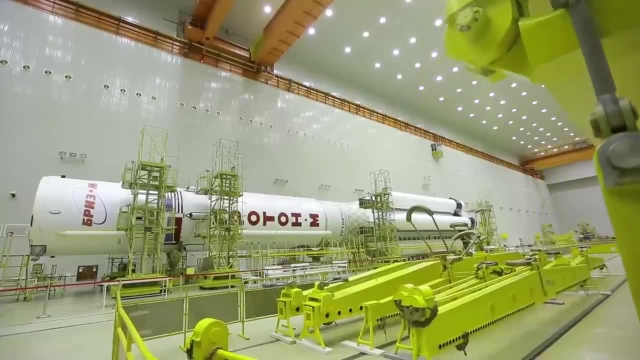 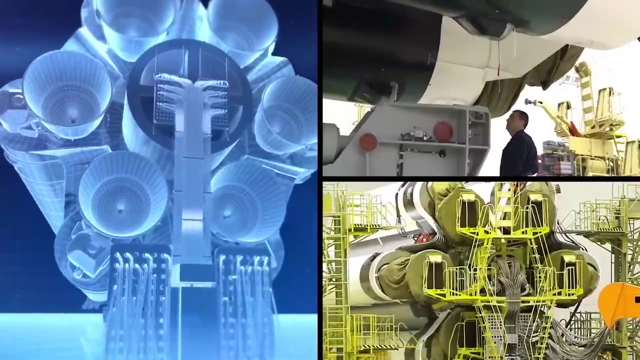 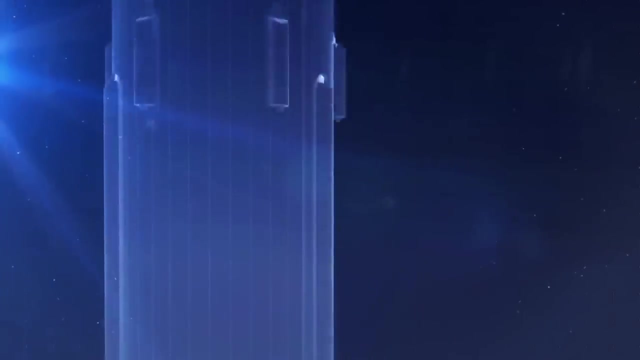 this is schematically depicted. in reality, however, takes a while to finish. the proton has already been fully assembled and tested at the factory. nevertheless, it undergoes a series of tests here as well. the proton is a heavy lift launch vehicle, meaning is more powerful than, say, a 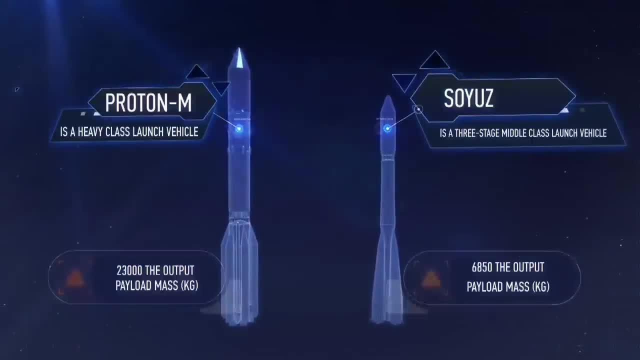 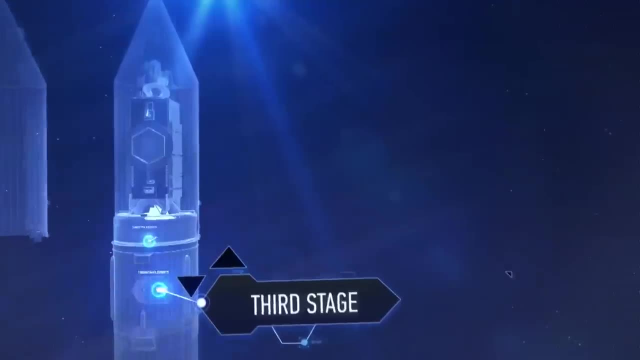 a middle-class rocket, Soyuz. Therefore it can bring heavier cargo into orbit. Proton rockets are three- or four-stage-to-orbit systems. The four-stage of the spacecraft is a booster And as a rule these rockets are used. 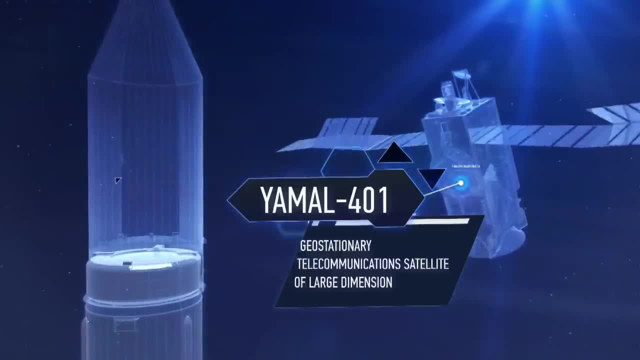 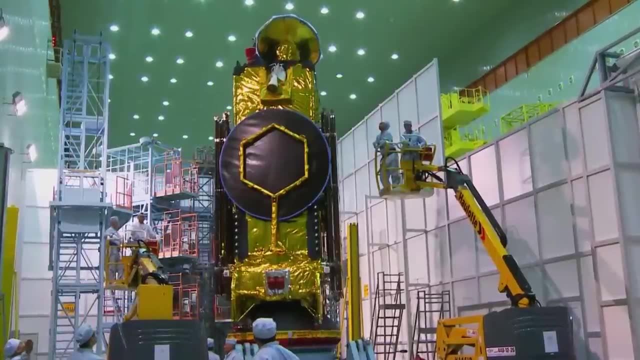 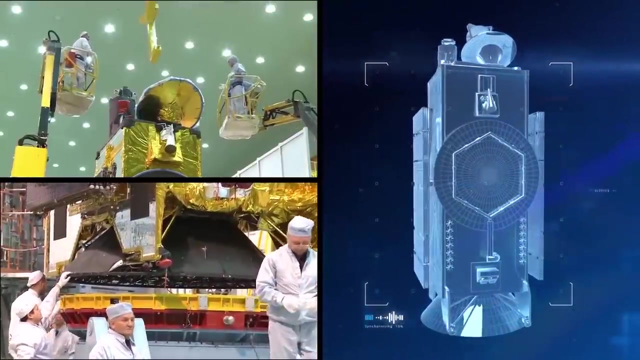 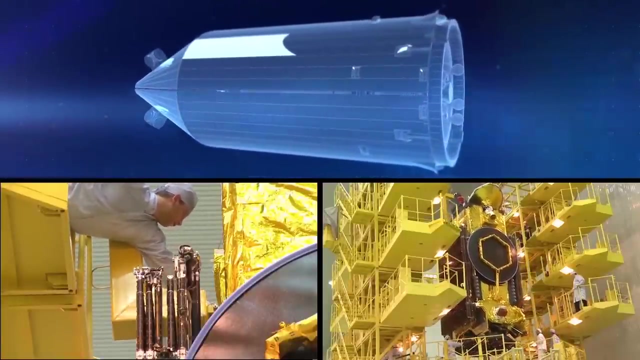 to launch geostationary communication satellites, the largest and the heaviest satellites of them all. The communication satellite is assembled and tested again on a separate jig. Now it's time to install the Yamal-401 to the rocket. The procedure is the following. 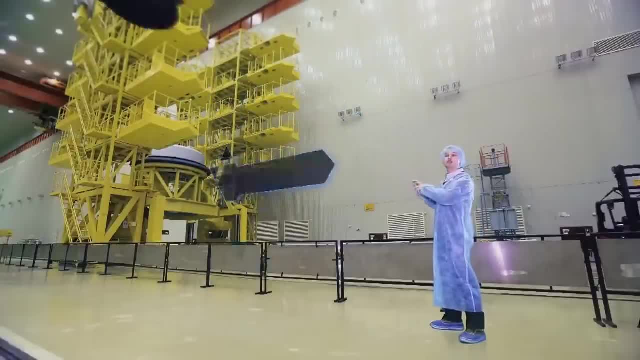 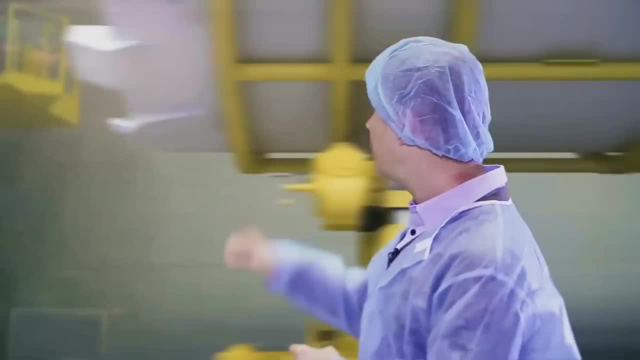 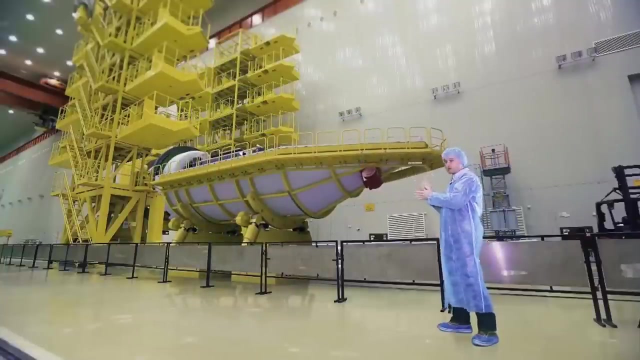 This jig locks the upper stage in an upright position, Then the crane lowers the satellite into the upper stage. Now they are joined, then inspected Afterwards. the first half of the nose cone rolls next to it and the upper stage along with the satellite. 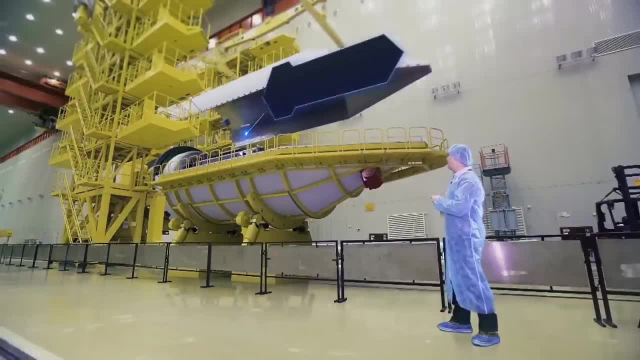 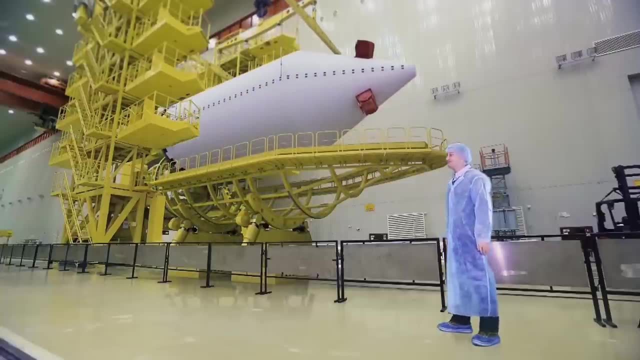 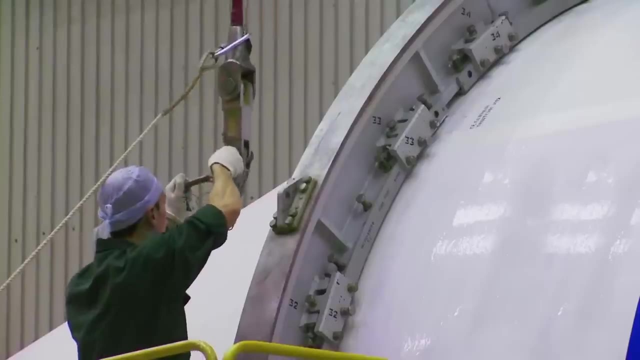 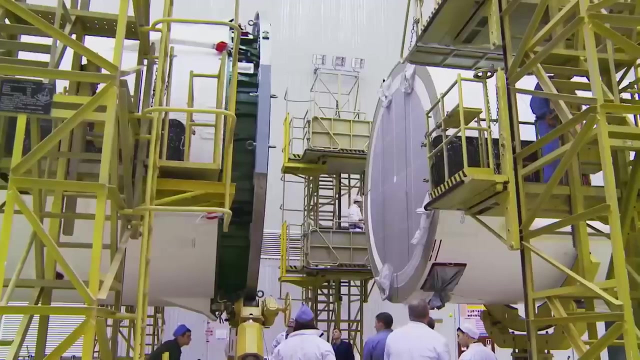 are lowered. The second half of the nose cone is lowered horizontally inside it. The structure is later sealed by the second half of the nose cone. And it's done. We're not nearly finished. The upper stage, together with the satellite, are later mated with the rocket. 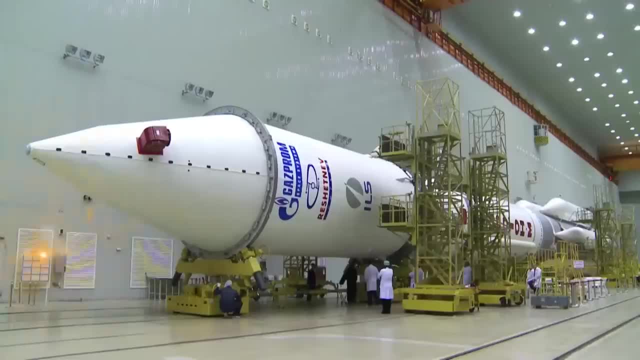 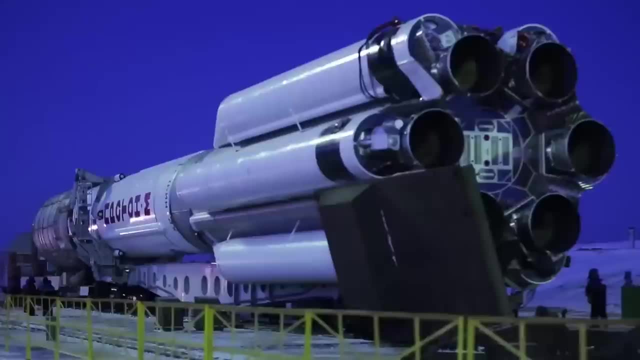 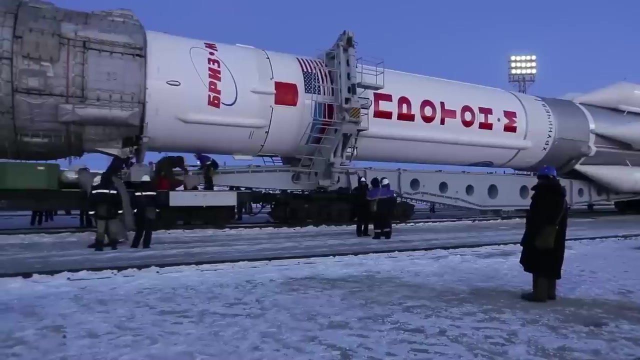 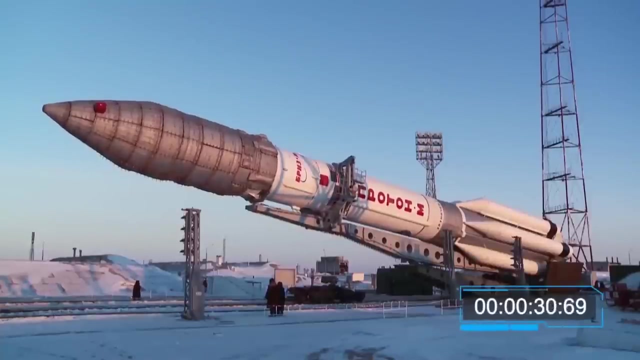 And so the LN launch vehicle is transformed into a space mission vehicle. We're going to prepare for a transplant, And more about this in our upcoming video. Proton is brought to the launching pad. It is detached from the rail transporter And placed in a vertical position. 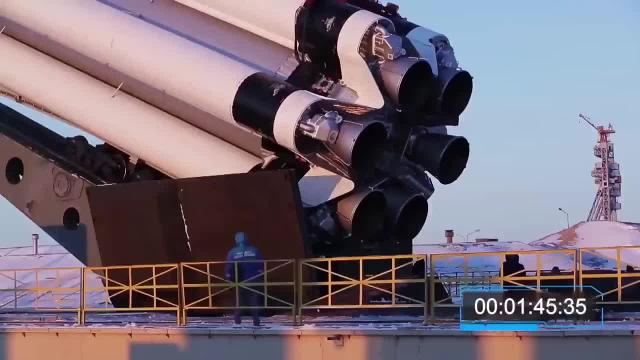 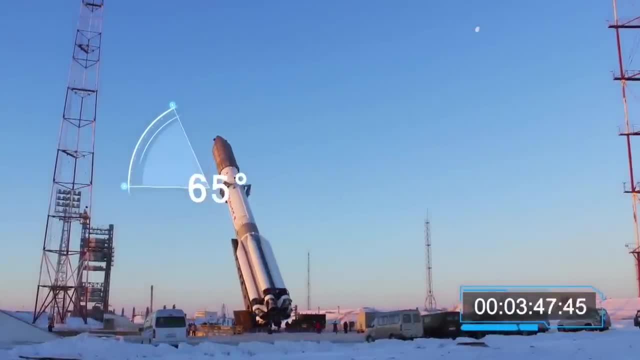 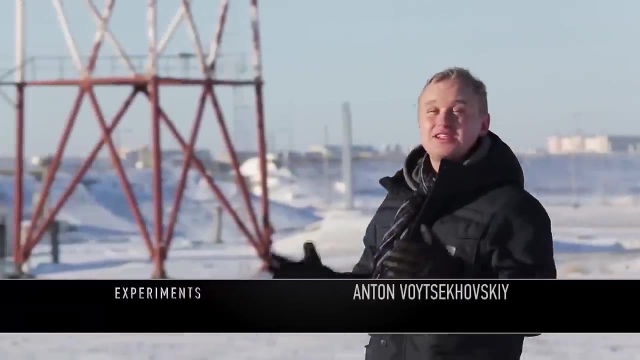 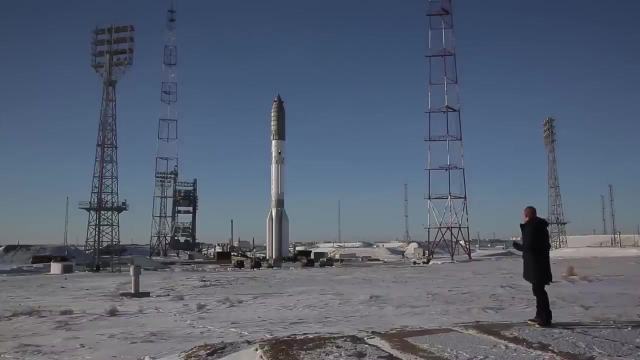 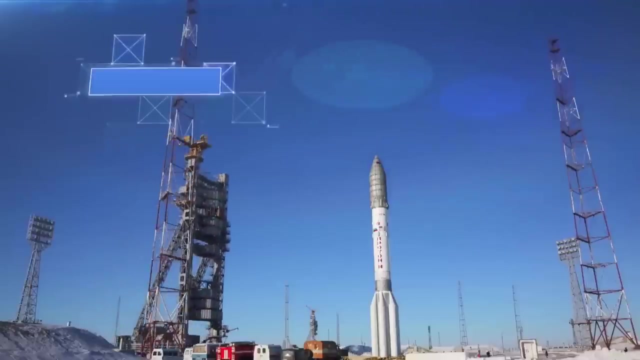 Saturn, Saturn, Saturn, Saturn, Saturn, Saturn, Saturn One would think. the rocket is finally here, positioned vertically and fueled, And now it can launch. But no, it's not over yet. The mobile service tower has rolled up to the proton. 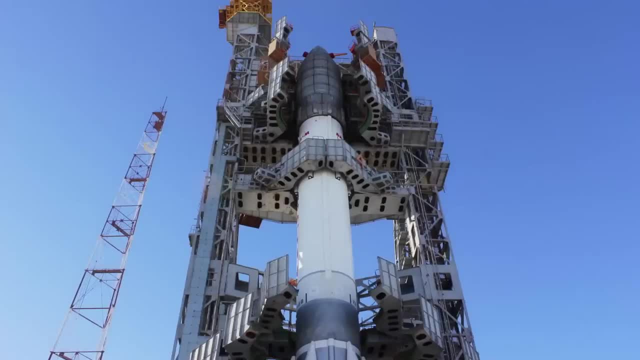 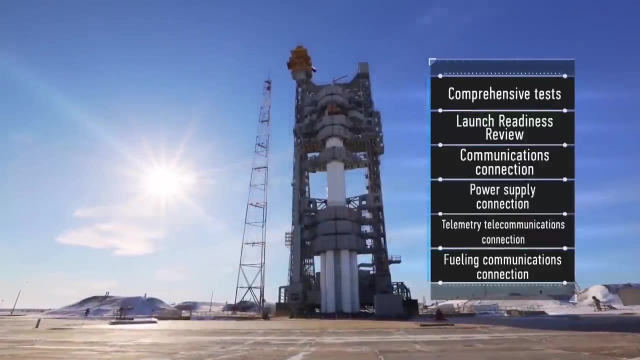 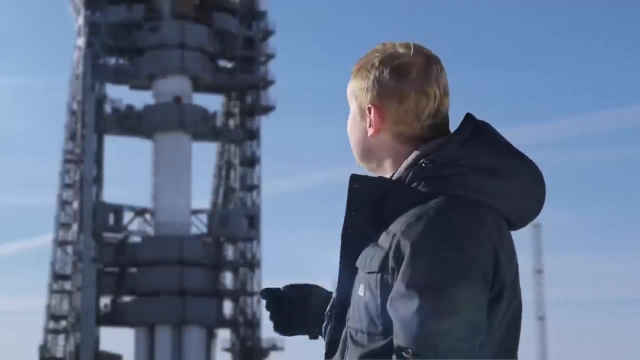 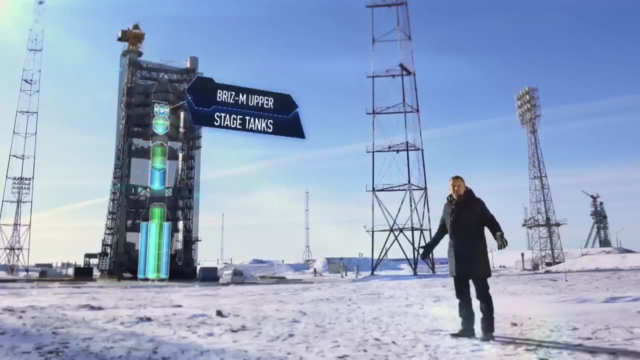 It literally embraces the rocket. There are still a few days left to launch. Fueling the rocket takes place on the fourth day. Oxidizer goes first, then fuel The first stage, the second, the third, except the upper stage because it has already been fueled. 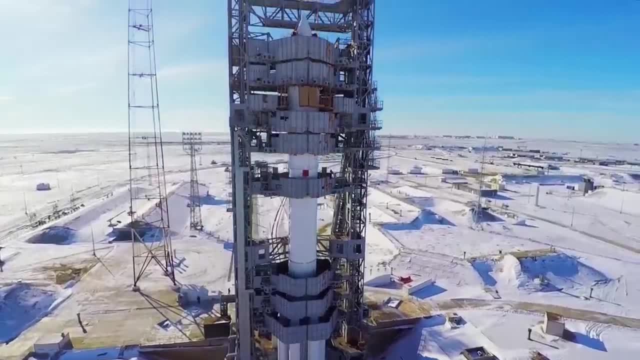 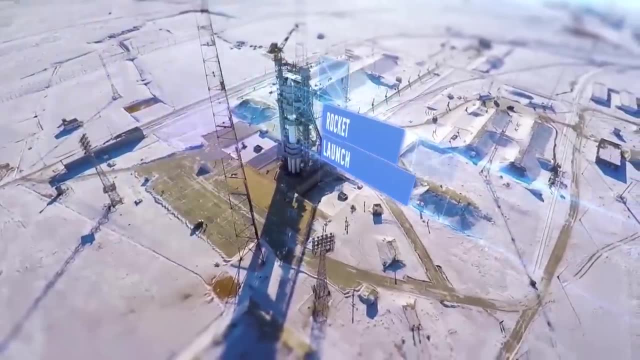 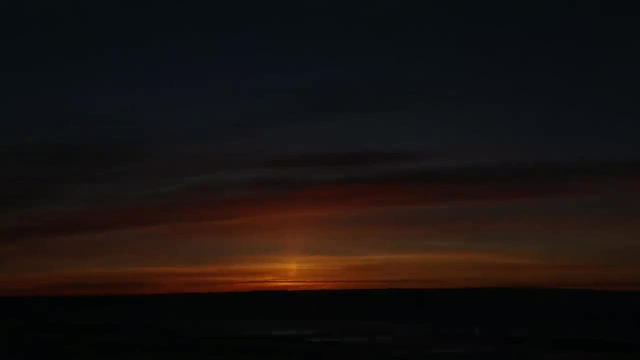 The launch usually takes place on the fifth day after the rocket has been installed to the launch pad. Now the question: will it launch during day or night? The takeoff of Proton M with the communication satellite Yamal 401 has been scheduled for early morning. 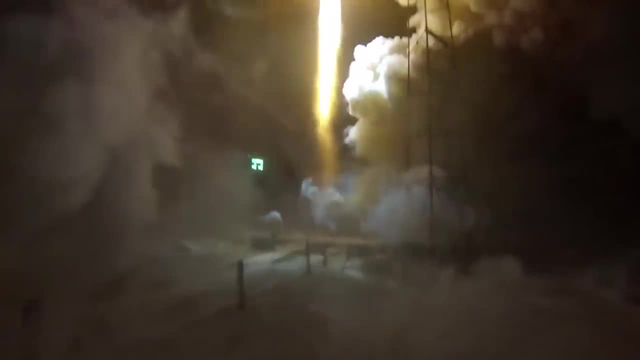 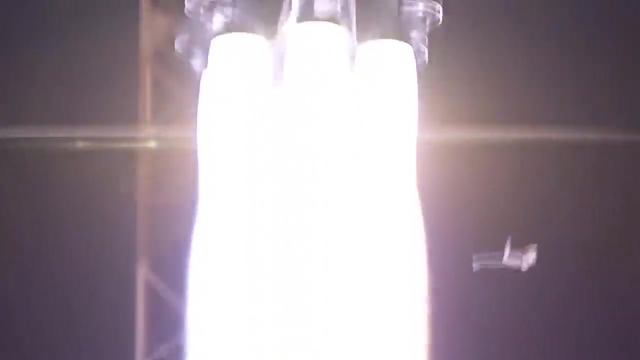 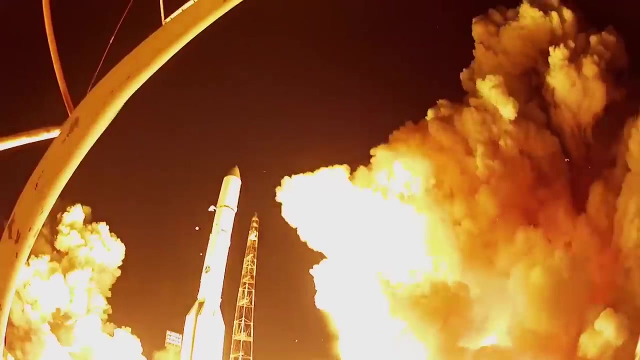 And I think in the near future theätzen try to carry a satellite Rochester engine. But in tat day before launch it's still going And NATO has already aired it Back to oriented series of tasks. The first goodbye was gonna be rocket-powered. 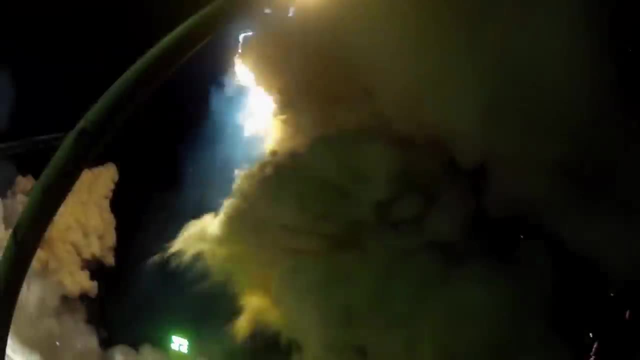 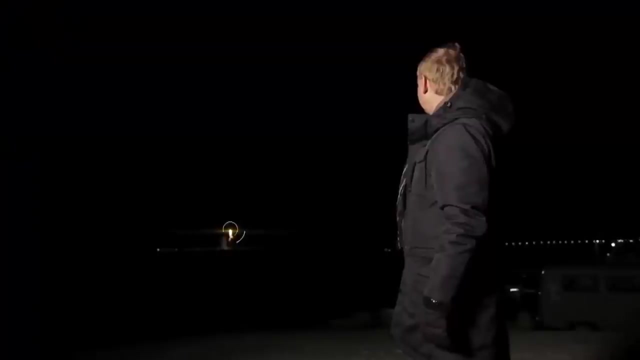 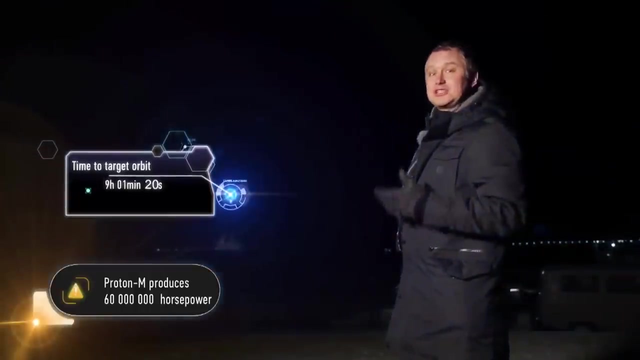 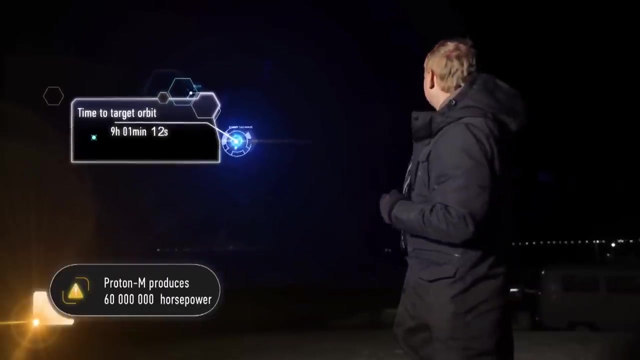 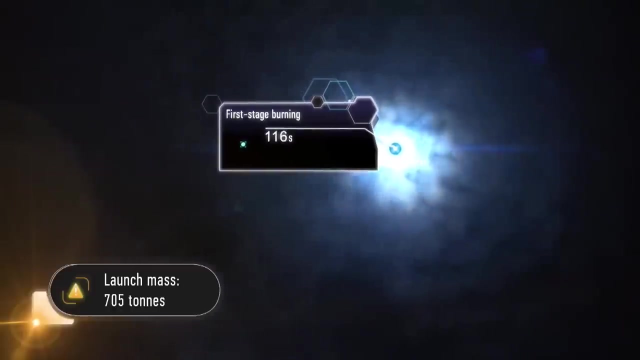 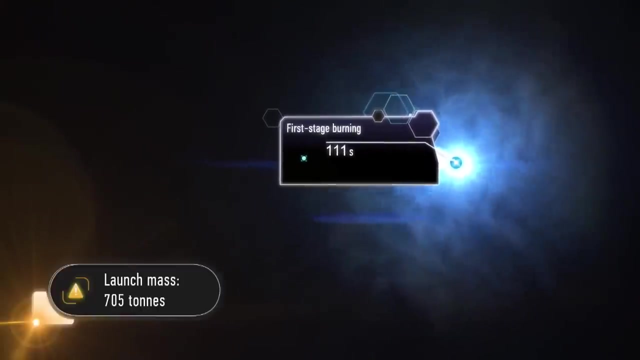 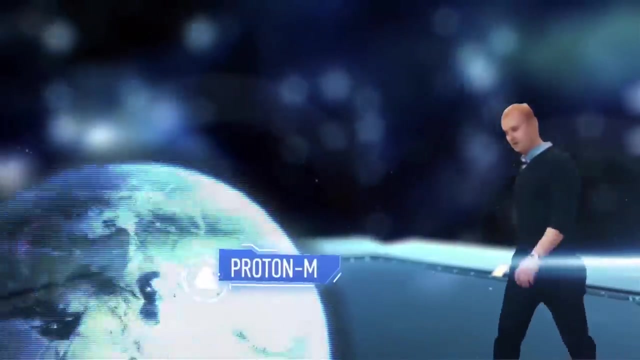 And then the second, realmente surprised, Since it came to contradict. The distance from here to the launching pad is about two kilometers, so the sound of the running engines comes with a delay. There it is, While watching the rocket launch or even stage separation, no one seems to wonder how. 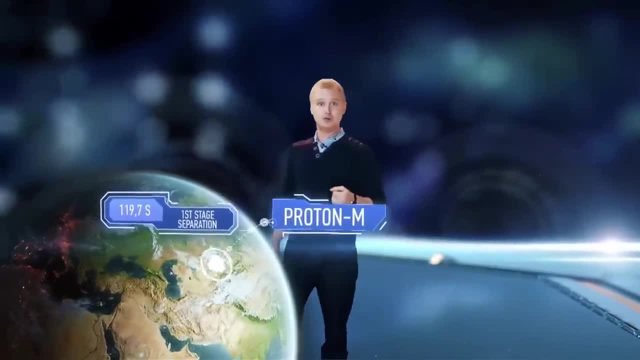 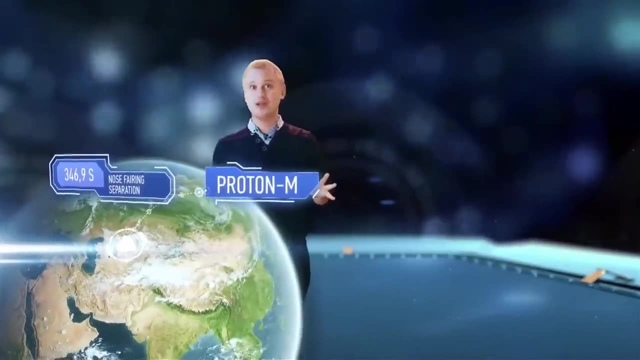 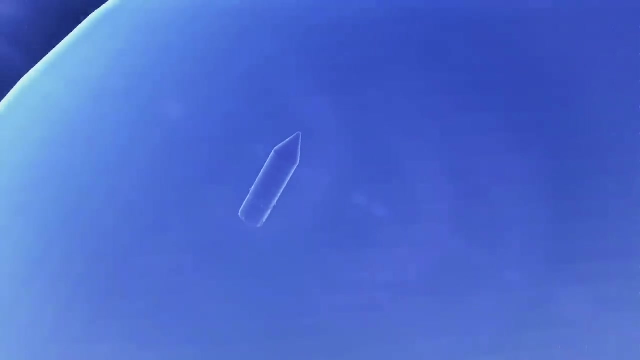 exactly the satellite reaches the orbit. It seems that everything is simple. It hits the desire. But no only when all the stages of the launch vehicle have burned out does the most exciting part begin. Three stages of proton push the satellite into the low or geosynchronous orbits. 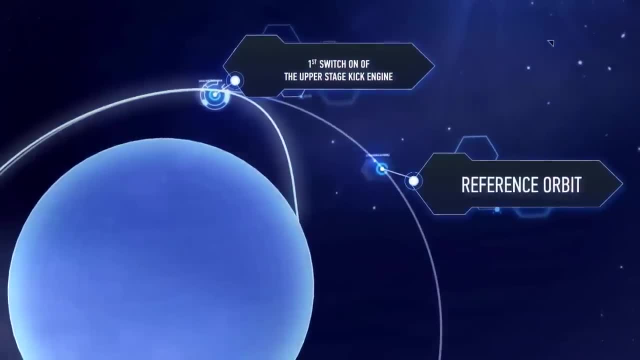 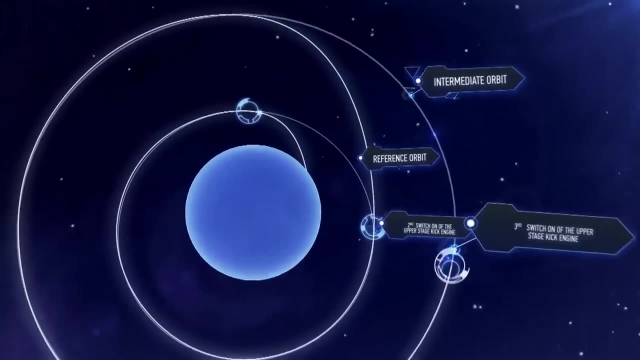 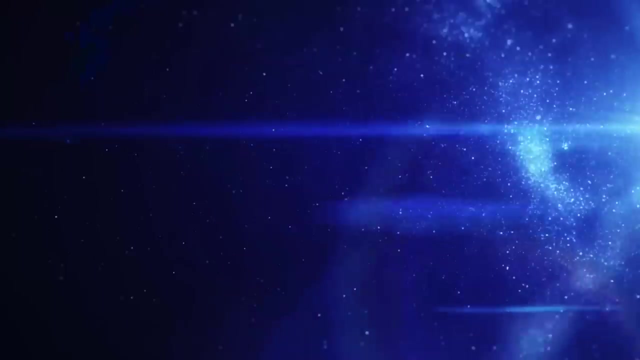 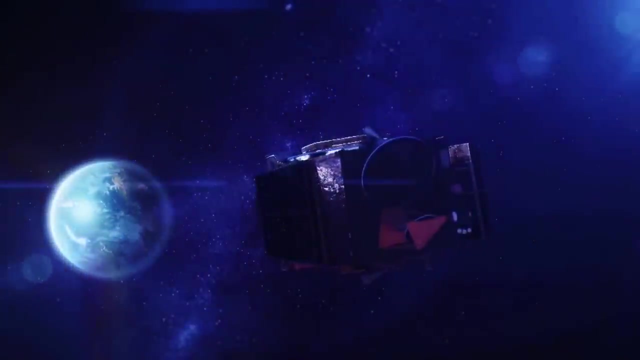 Then the upper stage starts functioning. It activates four times Each time the satellite accelerates to a new height and also changes direction. This is why the upper stage is also called the booster. Its job is far more complex. It takes nine hours for the communications satellite to reach the target altitude- 35,786. 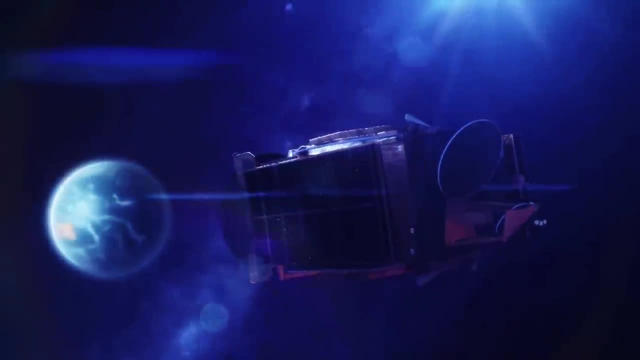 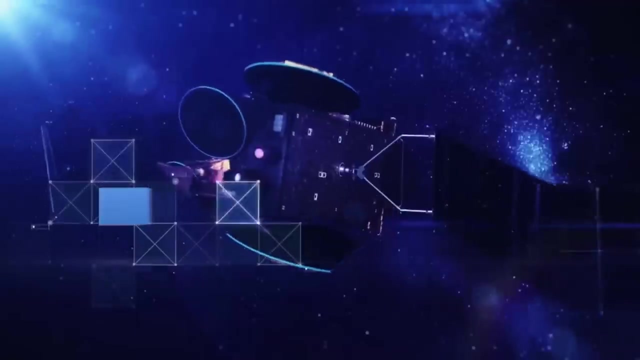 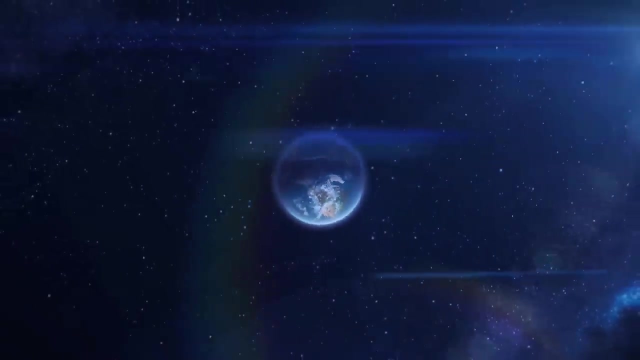 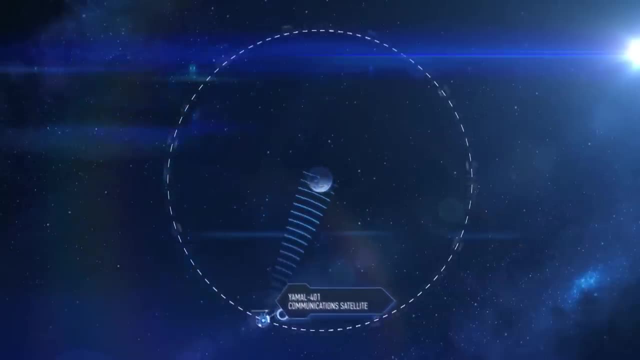 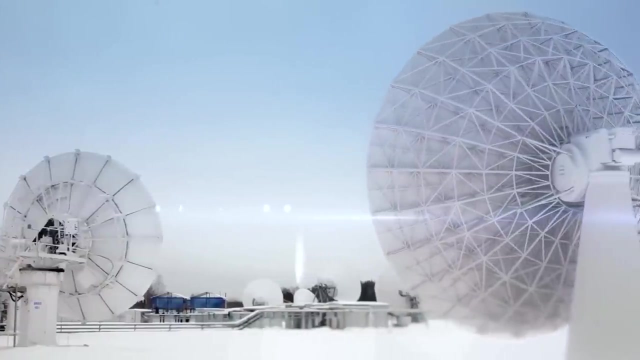 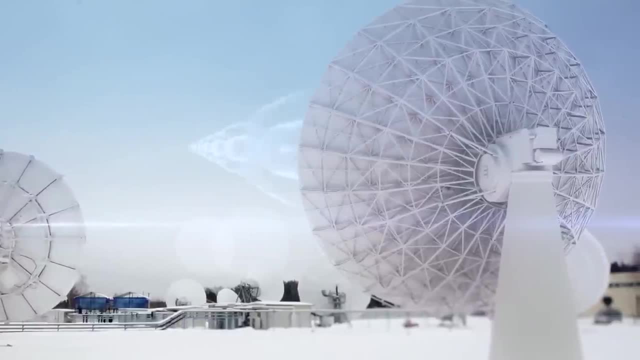 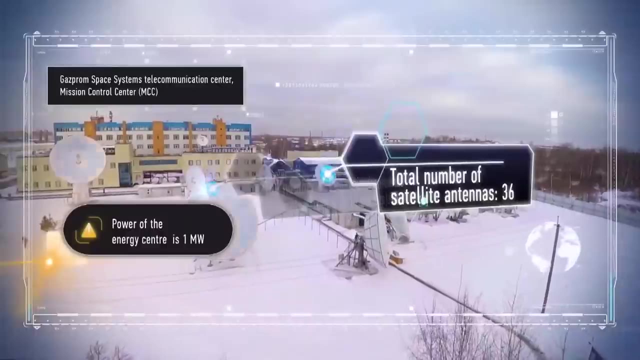 Constant reception. This, however, does not mean that there's no need to monitor the space-time as the planet It's. It's a very high-intensity station. It's high-intensity. That's why it's called a geostationary orbit. 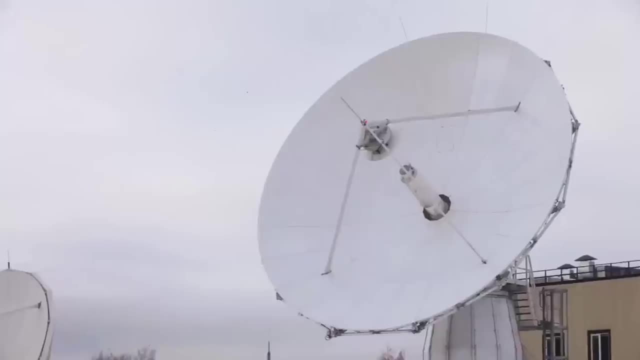 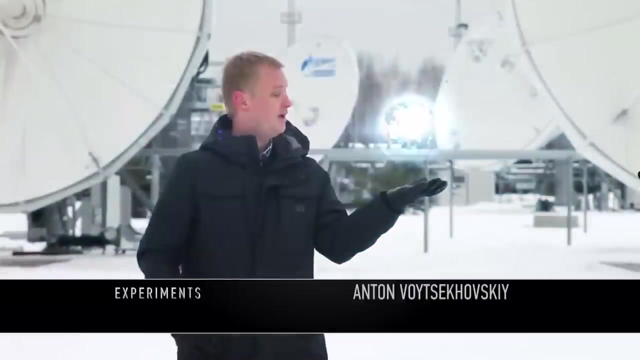 That's why it's called a geostationary orbit. That's why it's called a geostationary orbit to monitor the spacecraft's progress once it enters the orbit. Despite popular belief, voila, geostationary satellites aren't suspended perfectly relative to the Earth. 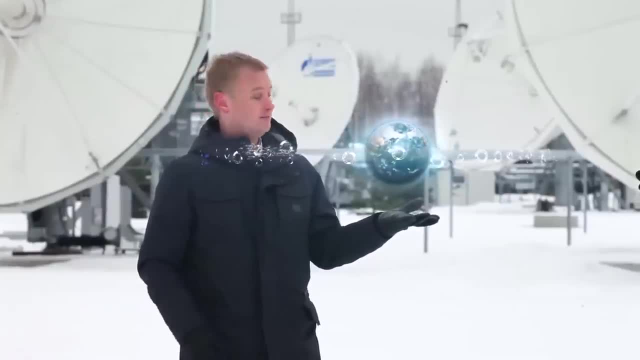 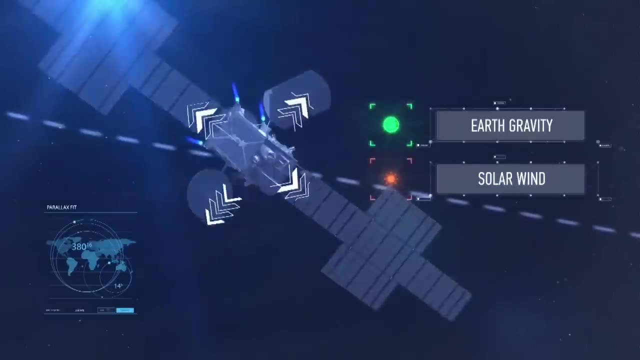 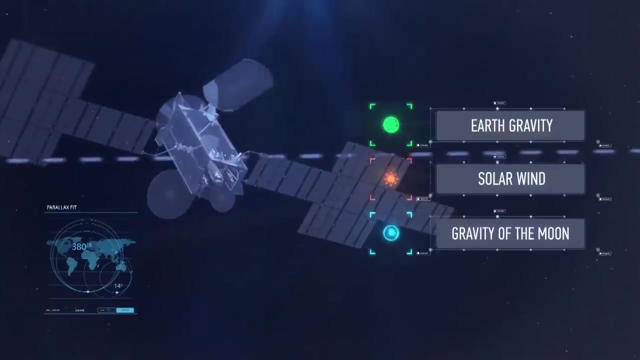 There are many factors that influence them, For example, Earth's gravity, solar wind, the gravity of the Moon. Each of them is trying to push the satellite out of orbit. Therefore, not only is the flight being supervised, but also thoroughly controlled. 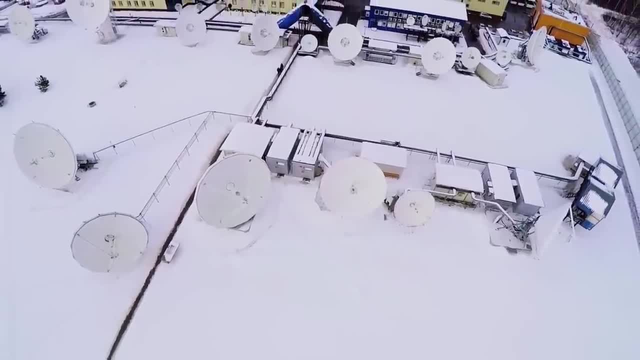 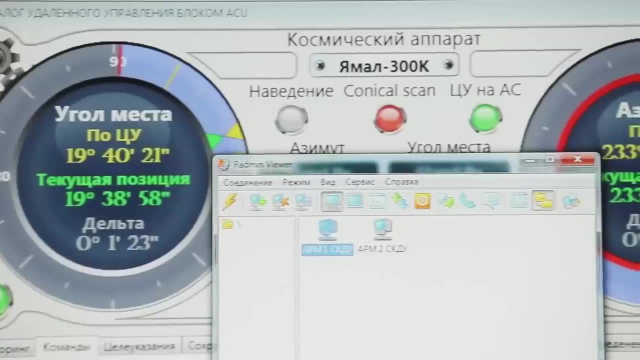 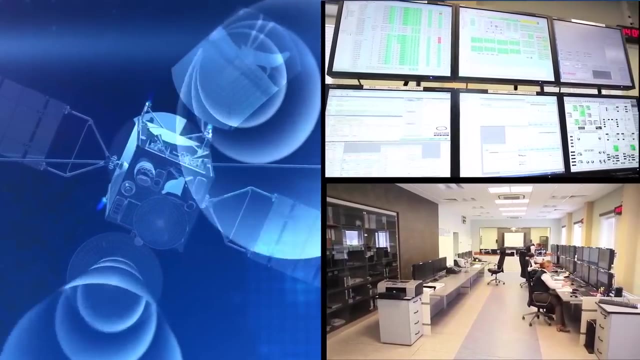 Control is being carried out by satellite operators such as, for example, Gazprom Space Systems. Here experts monitor geostationary satellite movements, correct their orbit, if need be, literally by turning on their engines to maintain them in their orbital positions.